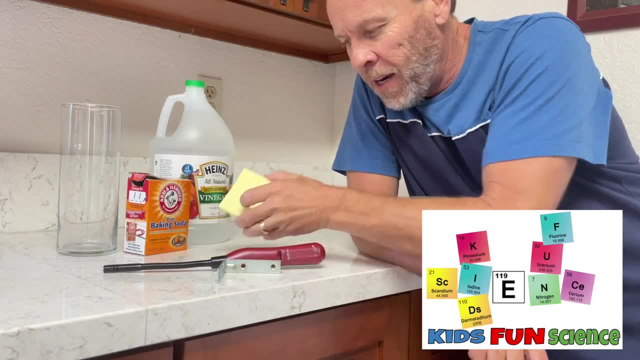 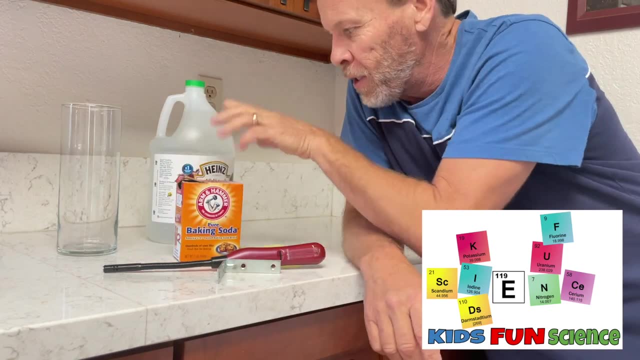 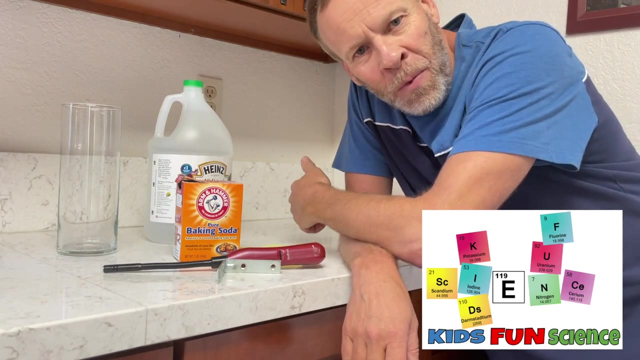 the world you're at. You need an L bracket and some of the stickies paper right there. Mine has stripes on it. It can be plain baking soda and vinegar, And we are going to make some carbon dioxide gas and we're going to float some smoke. So I'm going to show you how to do it and the 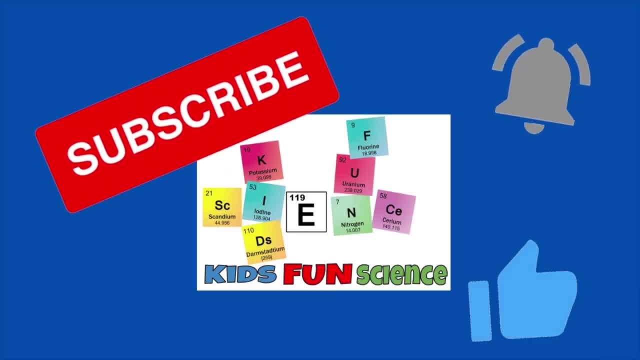 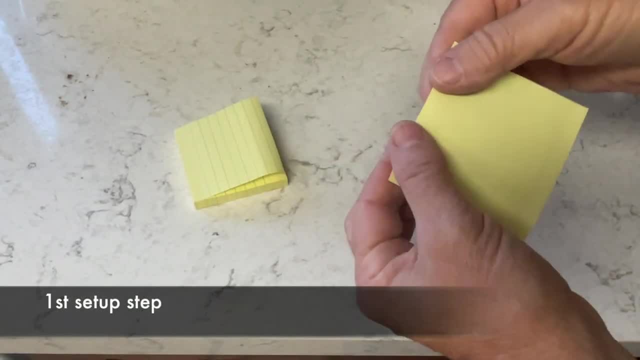 science behind it in just a second. Please remember to click subscribe and the notification bell and thumbs up if you like this experiment. So you take your sticky notes and you're going to roll it up with the sticky end on one end, but you want to make sure it's small enough to fit inside the 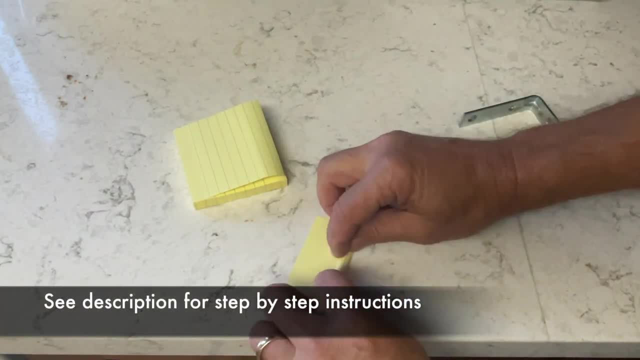 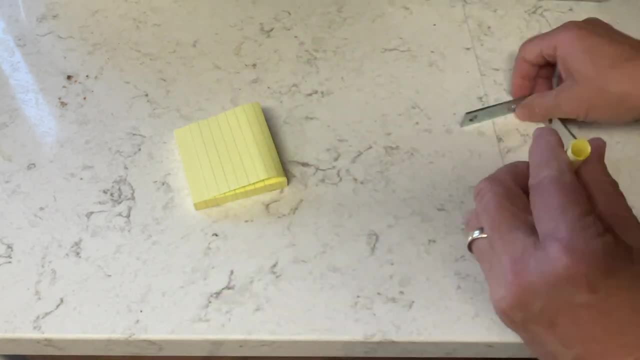 hole of the L bracket that you have. So when you're doing this experiment, you're going to rolling on the back side of the paper. When we get to the end, that's the sticky part and it should hold that in place right there, And now you're going to want to be able to be able to put. 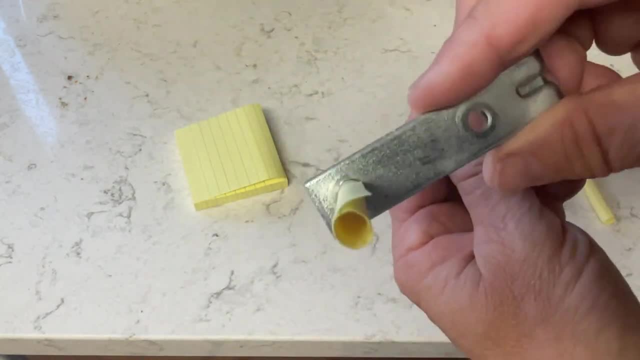 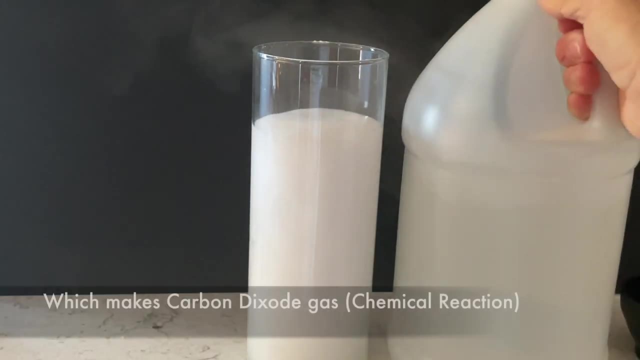 it into the L bracket hole, just a little bit in on the inside there. The second part of the experiment is: I have baking soda on the bottom of the jar, I pour some vinegar in and it creates a chemical reaction. It creates carbon dioxide, right. So now we have a gas inside there. So when 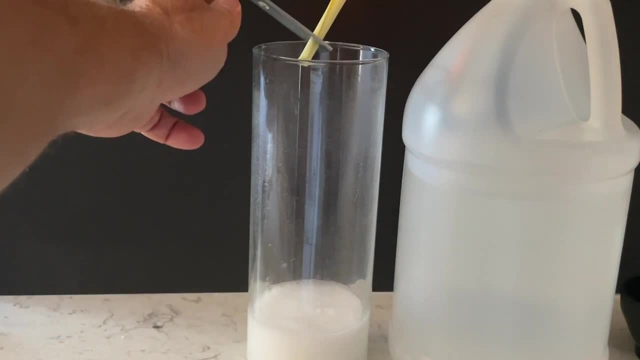 we have our sticky note hanging above and we take our lighter. we're going to roll it up with the lighter or torch and we light that sticky note on fire. the smoke doesn't rise as you're usually used to like in a campfire or a house fire or forest fire. The smoke actually comes down the 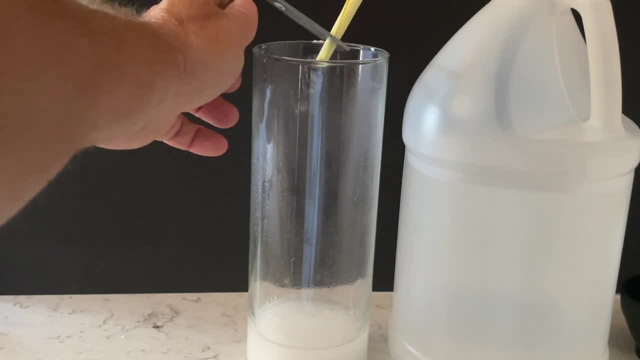 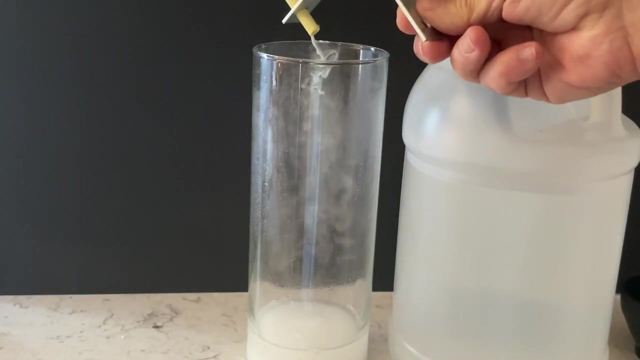 tube and goes down and falls to the ground, which is not normal. But the reason this happens is the science behind it is because the smoke has time to cool down inside the tube and therefore it's not hot and doesn't rise, and it sinks to the bottom or into the middle of the cup, as you can. 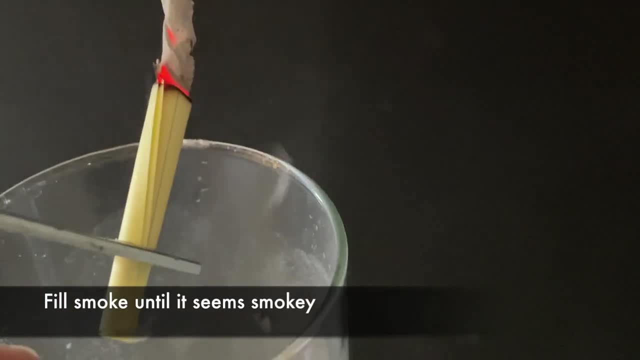 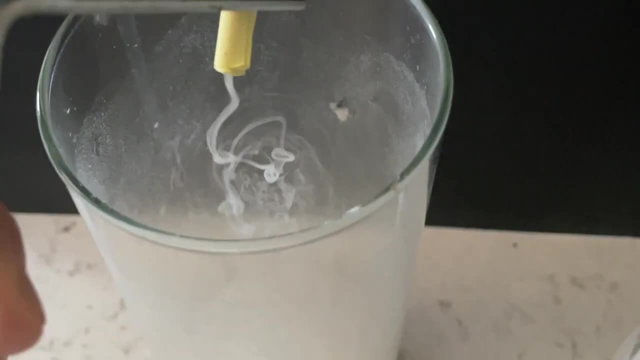 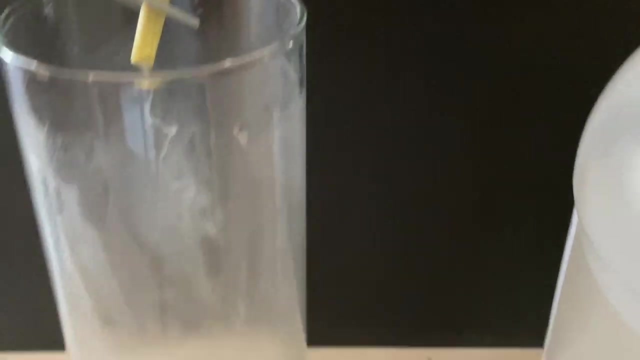 see here, Which is pretty cool. So now you keep letting it go a little bit. Be careful, because it is on fire there. Don't go too low. It will put out the fire because the carbon dioxide will kill the fire. That's why I have it above the glass. And now you see, you have this great smoke solution. that's kind. 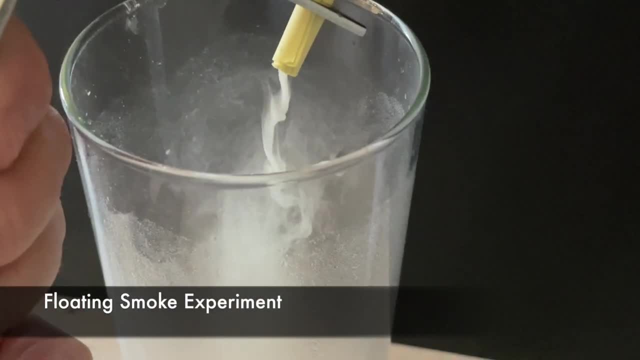 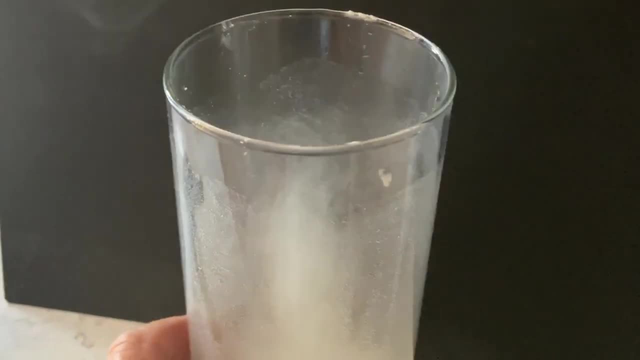 of just hovering in the middle of the glass. And this is where the science experiment gets really cool, because once you're done, you put the paper off to the side and you start shaking it and it's kind of like a liquid.